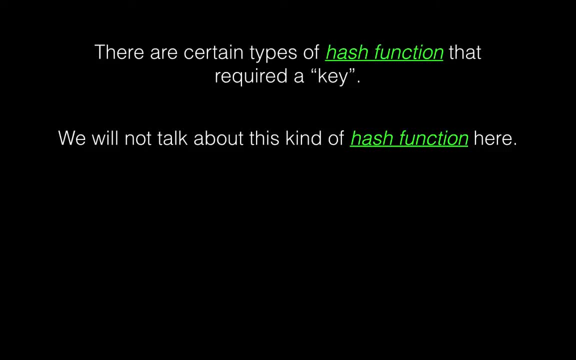 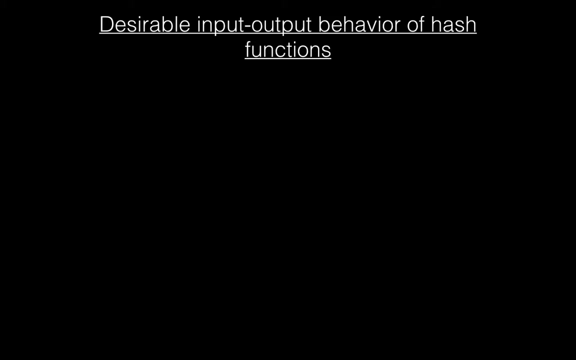 we won't talk about those here in this topic of hash functions. So every time I say hash function, I refer to the ones that have no key or are unkey hash functions. So the only input of the hash function would just be: whatever the data you want to transform into a fixed size, All right. so one of the things that we want to talk about is what are the desirable inputs and outputs? 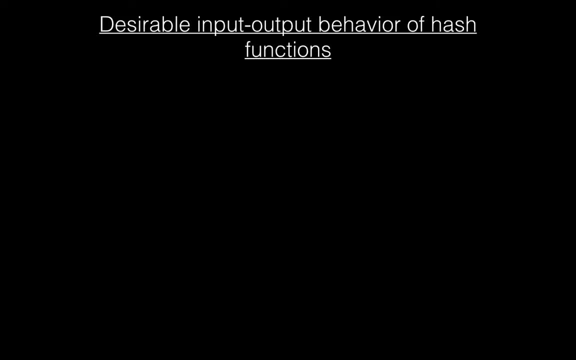 of the hash function. So what do we want the input and the output to be? So there are three basic things we have to consider. One is compression, The second one is easier computation And the third one is sensitive to all input bits, And I will go over each one of them in this video. So let's start with compression. So what is compression is is actually something that we already talked about. you take an. 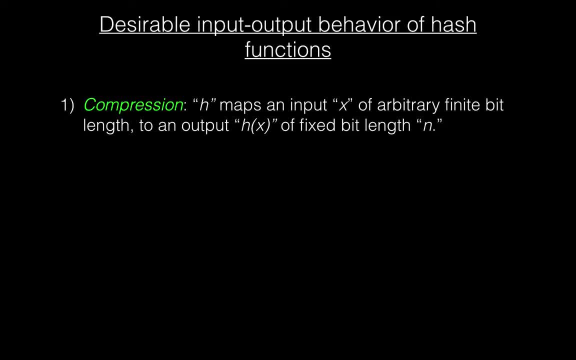 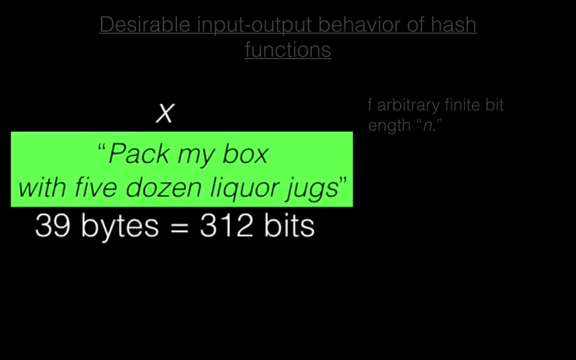 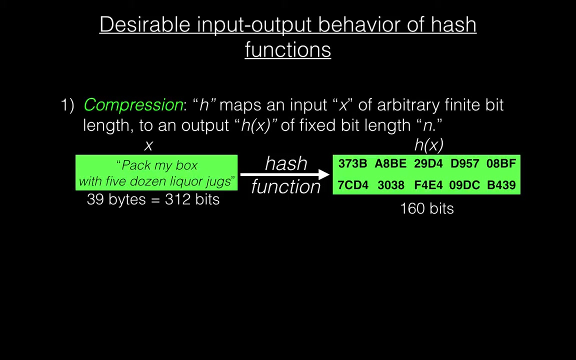 input of arbitrary finite bit or size And the output is a fixed bit length. So just to go back to the examples we did in the previous video, So remember, we had this string of characters pack my box with five dozen liquor jugs, which is about 312 bits. If I take a particular hash function, so that will give me 160 bits And this particular hash function is going to transform everything into 160 bits. So is you're going to 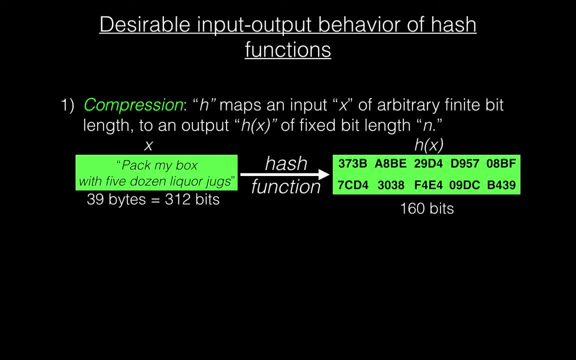 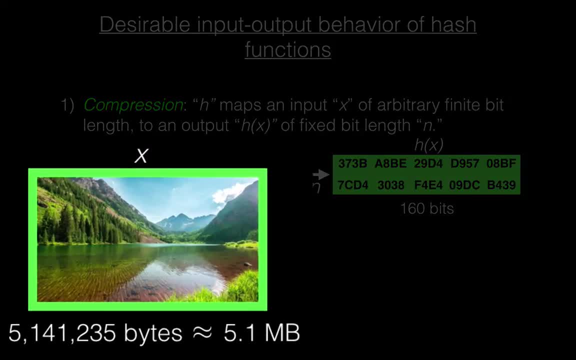 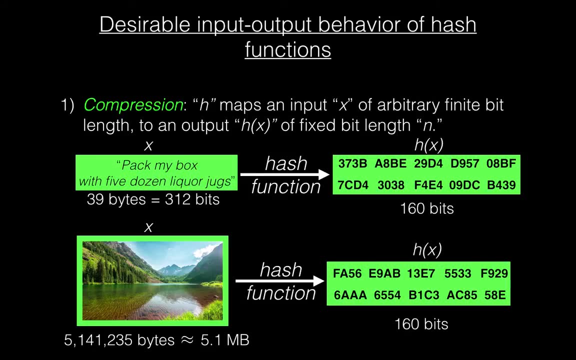 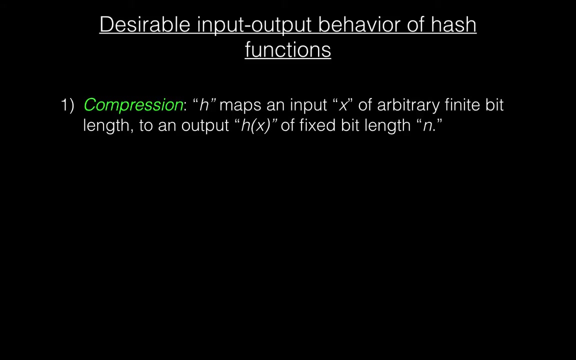 think about. that is the compression. So it compresses all that 312 bits into 160 bits. In a similar way, with the example of the picture, which is about five megabytes, I apply exactly the same half hash function and I will get exactly the 160 bits. So that's the compression, So something that actually is just a part of the definition of the hash function. So that's that part: compression. Now, one thing that we 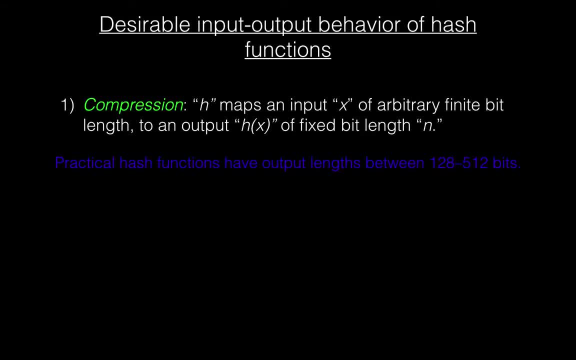 there is very common in hash function is that the outputs or the fixed size are usually between 128 to 512 bits. So all the hash functions that we will talk about here will have that range. that will be the output, the size of the output for the particular hash function. And of course there are lots of hash functions And depending on the hash function you will have a certain kind of output, like, for example, some of the hash functions will have: 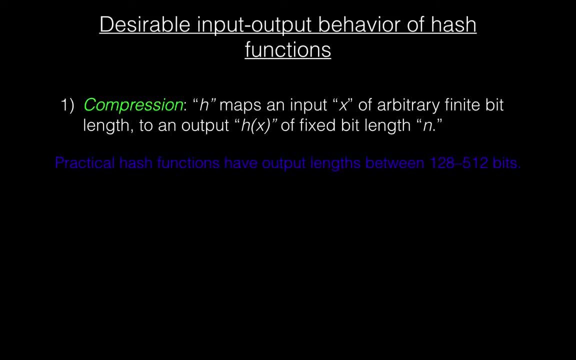 only 8 bits output. some others will have 160, and so on. So it just depends on whatever the hash function is. So those are the common values for the output. Now the second part is easy of computation. So what it says here, if you take an arbitrary input, call it x, the output h of x, which is applied the hash function to that input, is computational feasible. So there's not much I have to talk about. 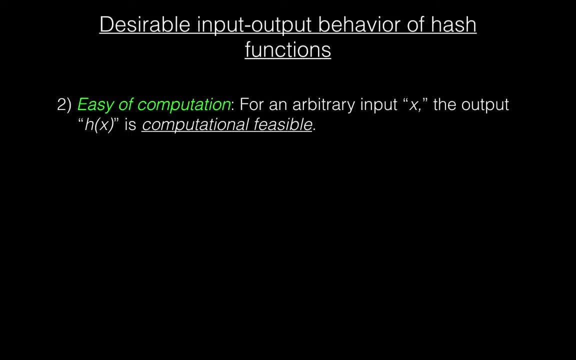 computationally feasible. it has a very formal definition but for us, for the moment we're going to talk about computationally feasible is that you can actually compute it in a reasonable amount of time. so that hash function should be, let's say, easy to compute. so if you give it any input, it 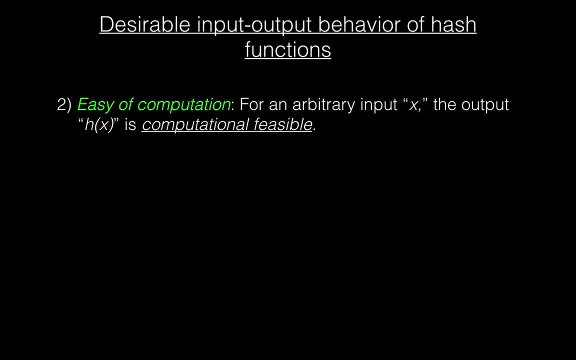 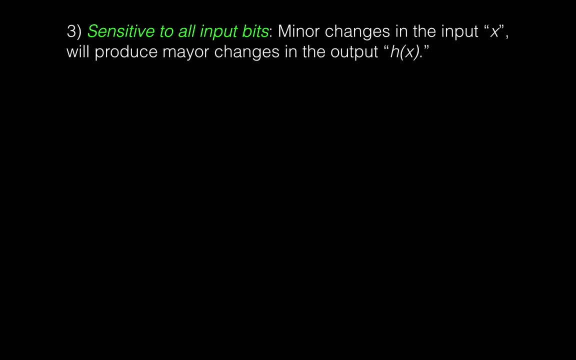 doesn't matter how big or small the input is. the output, or applying the hash function to that input, should be easy to compute, so should not take too much time. now. this is also very important and is sensitive to all input bits. so what that means is the following thing. if i change a little, 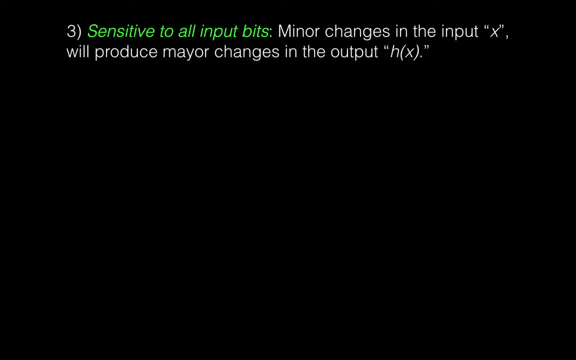 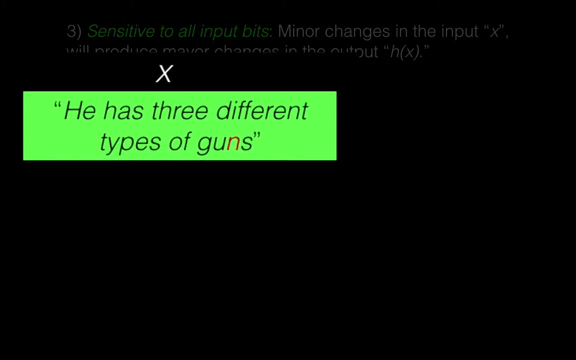 bit the input x, just maybe by one bit or one byte, that will produce a major change in the output of the hash function. let me explain that with an example. so let's say i have here this uh string of characters and which call that x. so he had. so the string of characters is he has 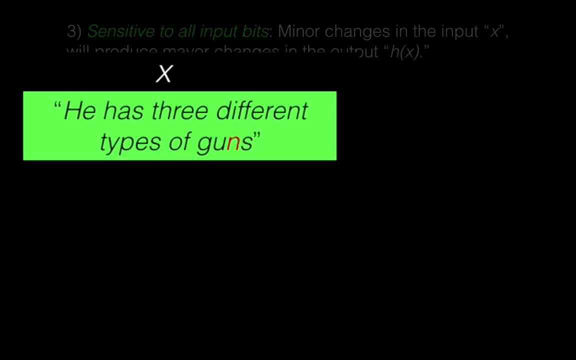 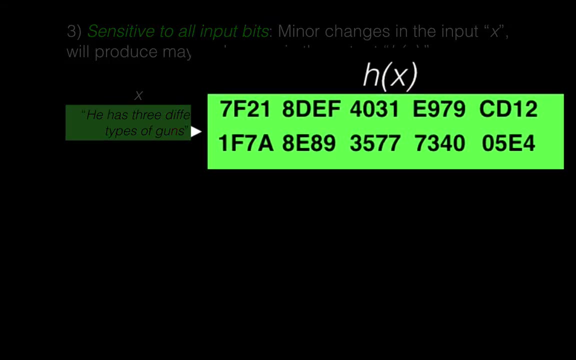 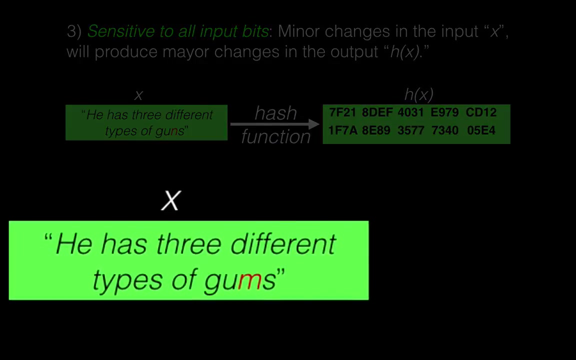 three different types of guns. now, if i use a particular hash function, i will get that output that you see there. now let's consider something that is very similar to that string of characters, which is the one i'm going to show you now. he has three different types of gums now, if you notice, 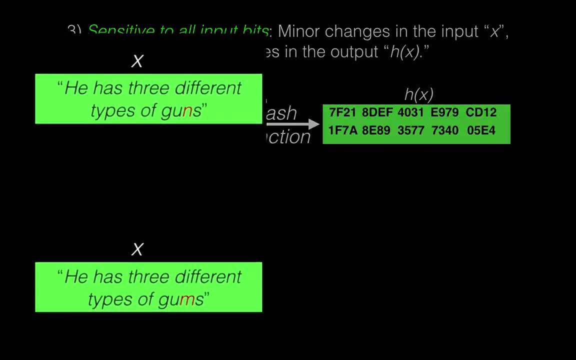 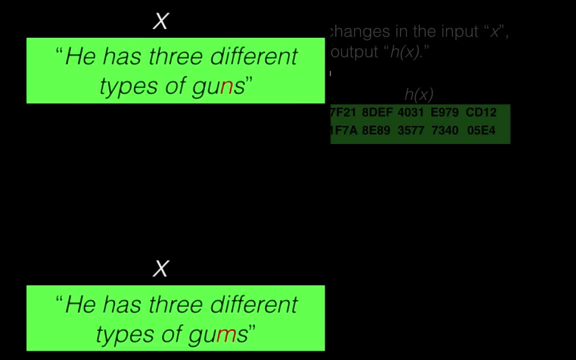 uh, the two different, uh, string of characters. they differ by only one letter. so if we think about this letter represented as, as a byte, so basically what we are saying is that these two strings just differ by one byte. now the result of the hash function should be different, because 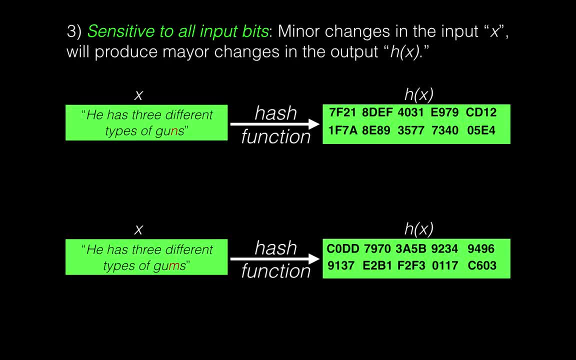 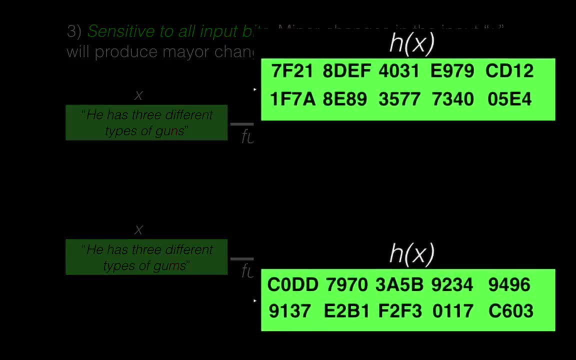 it has to be sensitive to all input bits. so if i apply the hash function, as you can see there, the output is actually completely different to the output of the first string of characters. So just a little change in just one letter, just eight bytes, or sorry. 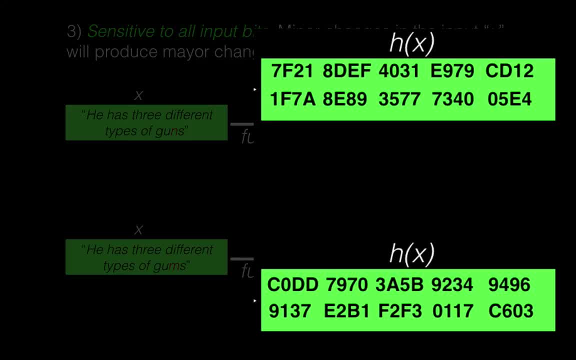 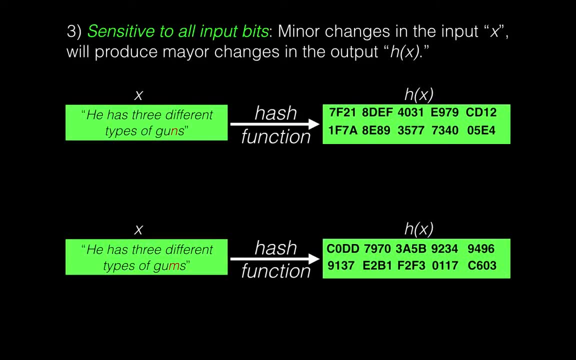 one byte, it will give you a completely different output, And that's one of the things that you want in a hash function. Now, that's for basically security reasons, And we'll go into more details on why we want all these kinds of things in the hash function. So that's the input output behavior. 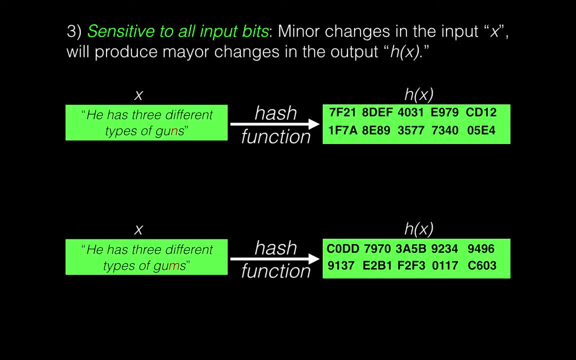 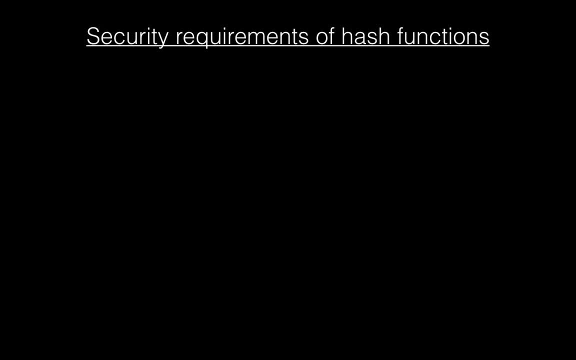 we want. So we want three things. that the one we went over already here. Now there are also some security requirements of hash functions. Now remember the ones that we're talking about here. they do not have keys. So there is more. there must be some way to secure the hash function. 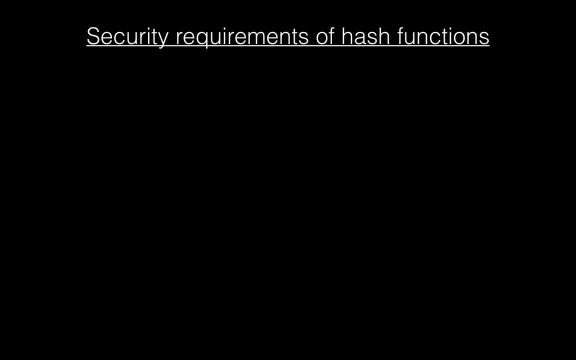 and secure in some sense, that I'm going to talk about in right now. So the first thing is called the pre image resistance, or one wayness, something that we actually talked about in the previous video. we talked about in the previous video, we talked about in the 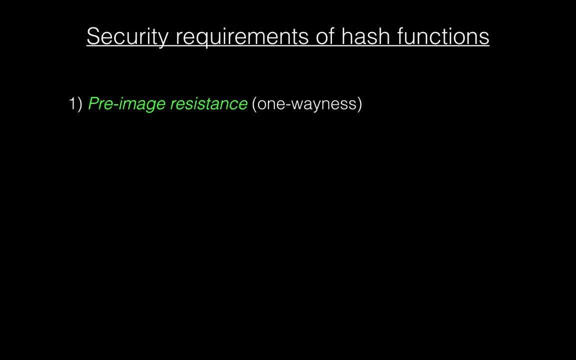 course already that's a one way functions, but we'll go over it This anyway. we'll repeat what that definition is. The second part is the second security requirement is that it's called second pre image resistance or is also called with collision resistance. And the third security. 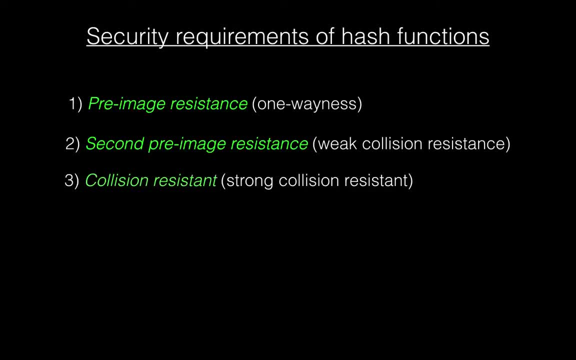 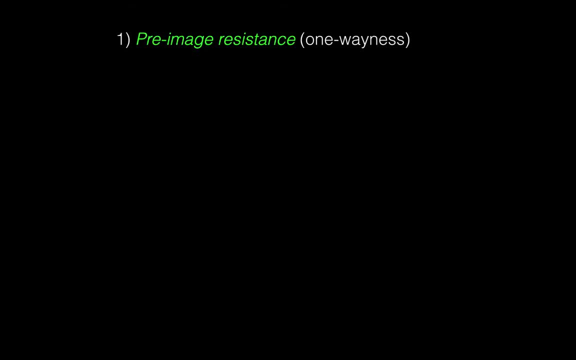 requirement is that you have collision resistance. in this case is also called a strong collision resistance. So let's go over each one of them. So what is this? Well, the first one is called the pre image resistance. is basically what it says is that a hash function should be a one way. 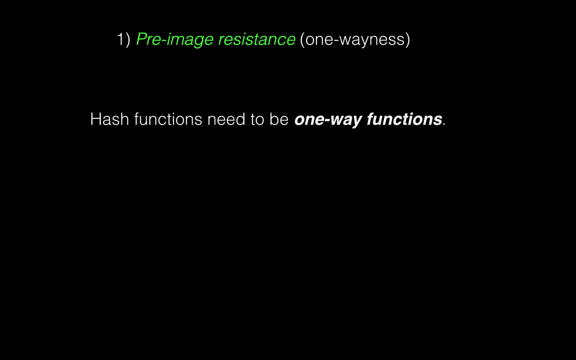 function. We talked about one way functions in this class already. That was an important part of cryptography. So basically, let's recall what that actually is. So what that is is if I give you an output that is usually between 128 and 512 bits, it must be computationally infeasible to find. 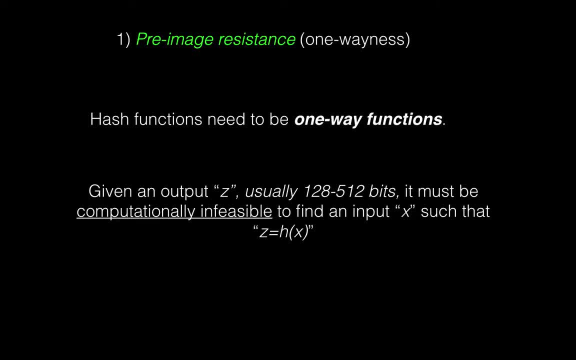 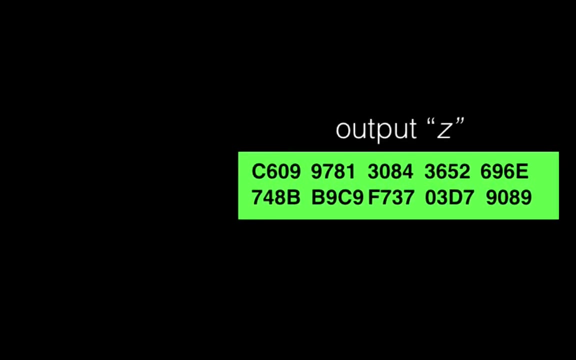 an input That maps to that output. So that's basically the definition of one way function. that is really difficult to invert the function. Basically, that's what the one way function means. So an example here could be something like this: suppose I give you an output which is that: 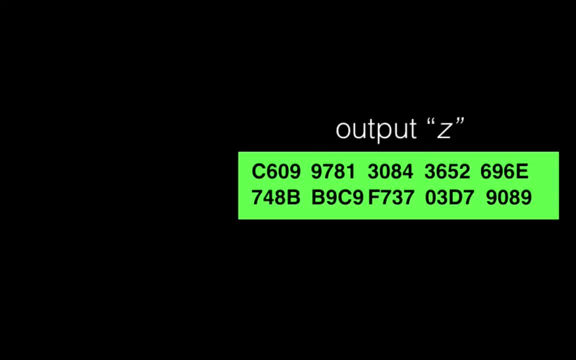 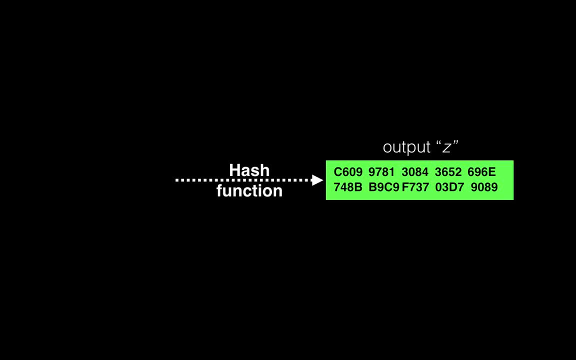 hexadecimal number that you see there, And then so one way function h, which is the hash function, should be a one way function. means that it, if you know what the hash function does, so you have actually the output. you know what the hash function does in general. so the general setup. 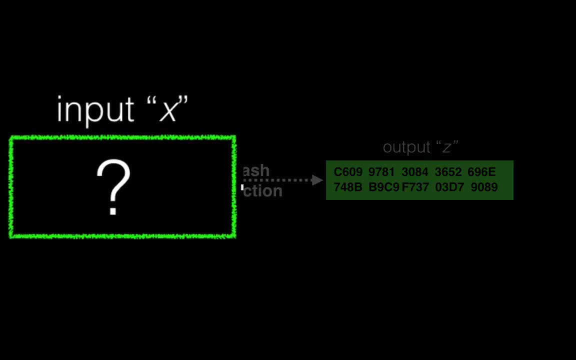 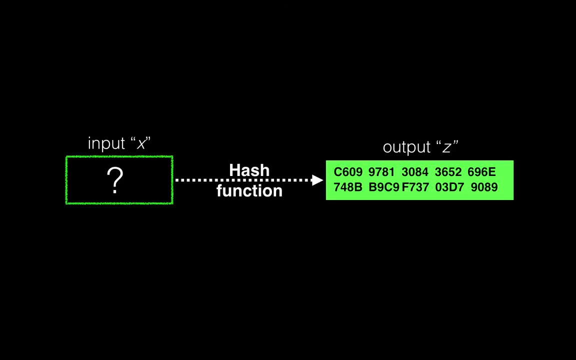 of the hash function. it will be really difficult to find an input that maps to that output, given that you already know that hash function. So now remember that this is also. this is exactly the same definition we had for one way function, So it's basically the same. So that's what I said. 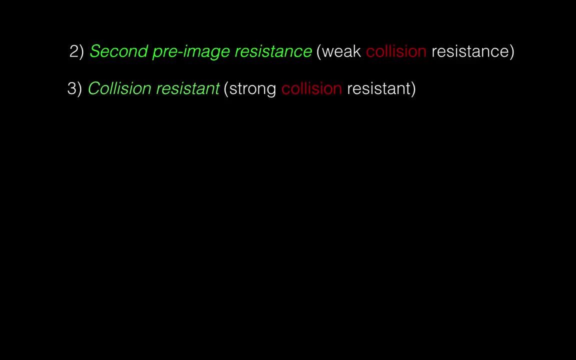 there's this: computationally infeasible. Okay, so we have two other requirements: the second pre image set resistance and the collision resistance. Now, if you notice, here the word collision is there, So I think it. I want to explain first to what a collision is before I go into number two and three. So let's just 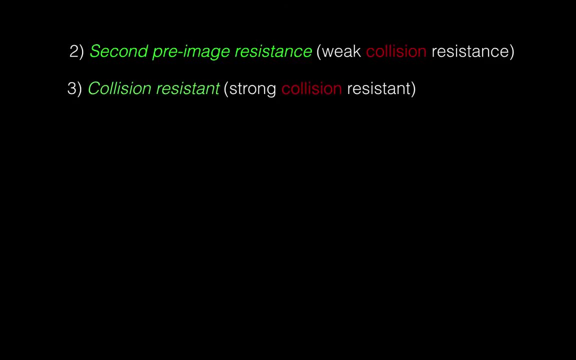 go over what a collision means in a hash function. So what is a collision in a hash function In general? what is a collision in any function? So we'll talk about hash functions in particular here. Now suppose we have a hash function that takes any input and and transforms that into 160 bits. 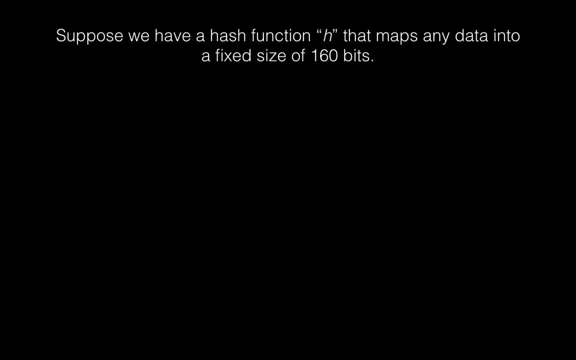 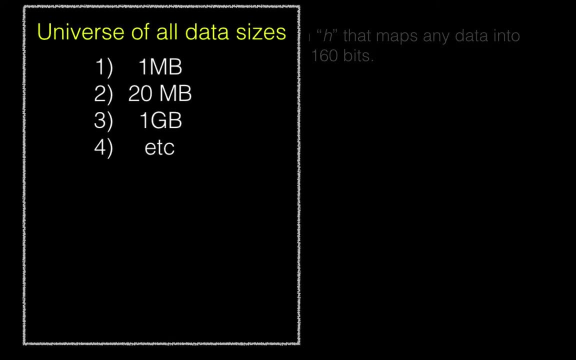 Now the hash function should be able to manage or to have inputs of any size. So if I think about the universe of all data sizes, so you have files, so, for example, one megabyte, 20 megabytes, one gigabyte, and you have a data files with data sizes that are longer than that is smaller than. 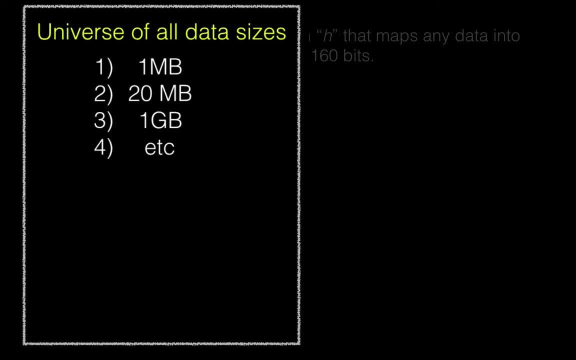 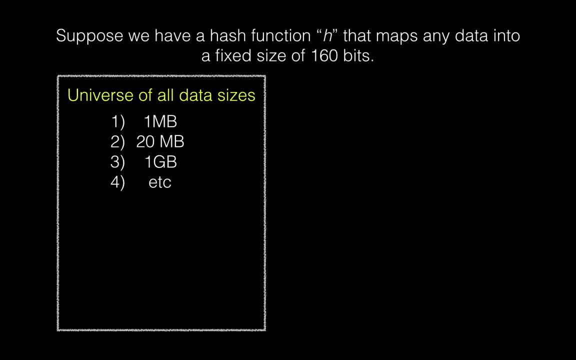 that of files. so there is a lot of them, actually tons and tons of them. now, when the hash function does, in this particular case, we want the hash function to produce 160 bits, so it's going to take all those files that you see on the left in the universe of data sizes and it's going to map. 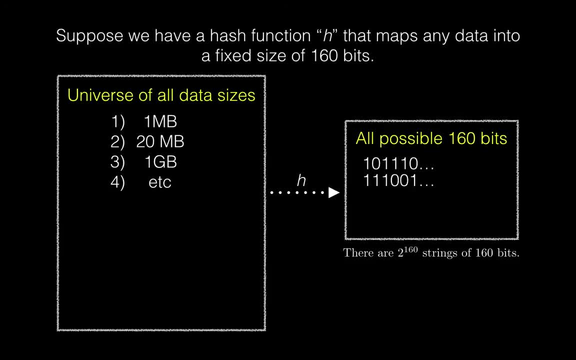 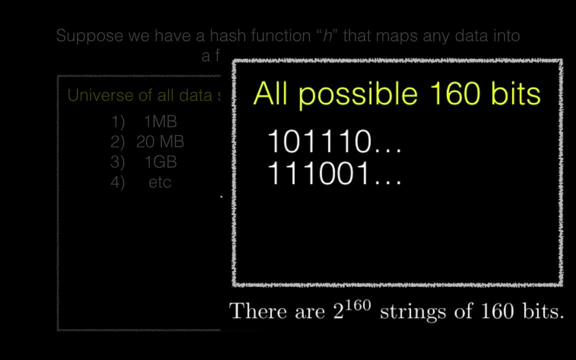 that into 160 bits. so the output is going to be 160 bits. so how many of those outputs are there? so how many possible 160 bits are? there is two to the 160.. if you think about it, you have 160 positions and each position could be a zero or one. so there's a. possibly there's two possibilities. 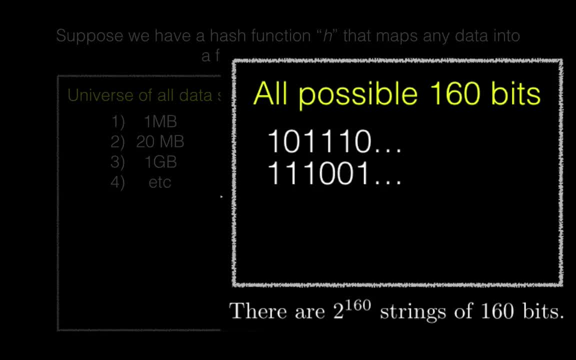 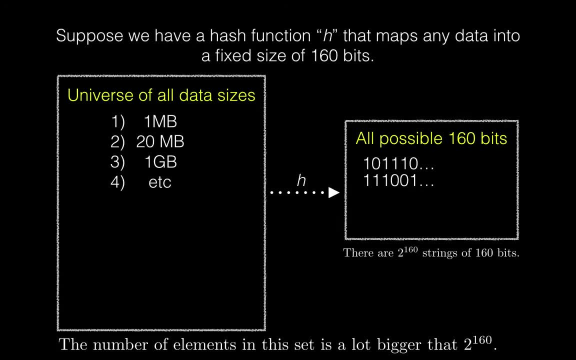 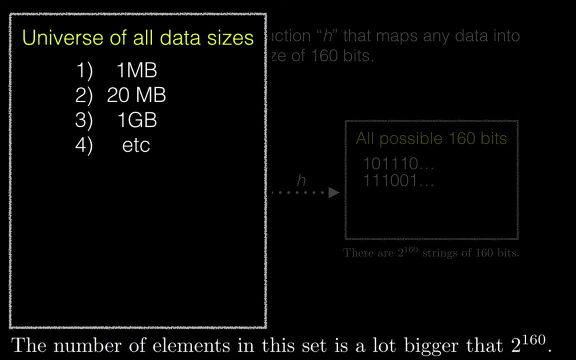 for one position. that's why you get two to 160.. now, two to the 160 is, of course, a really large number, but the problem here is that the number of elements in your data sizes and the inputs is a lot larger than that. so if you think about only the files that have one megabyte, there are a lot, a lot more files that. 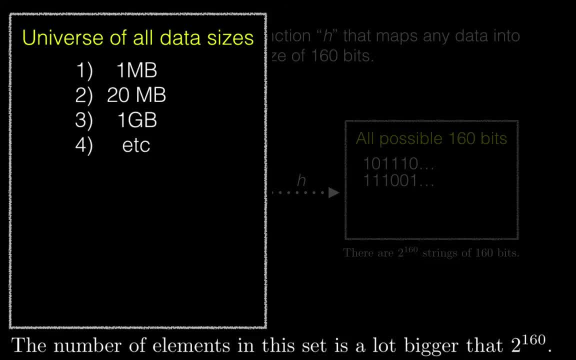 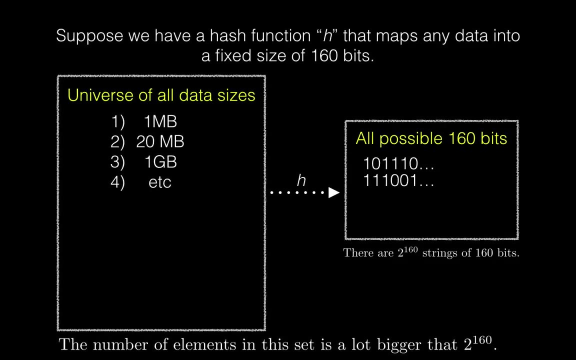 have one megabyte in size, that there are 160 bits, uh, strings of that size. so, because that is the, the, the difference between the input and the output, the number of inputs is a lot bigger than the number of outputs. there must be at least two distant files that have the same hash. 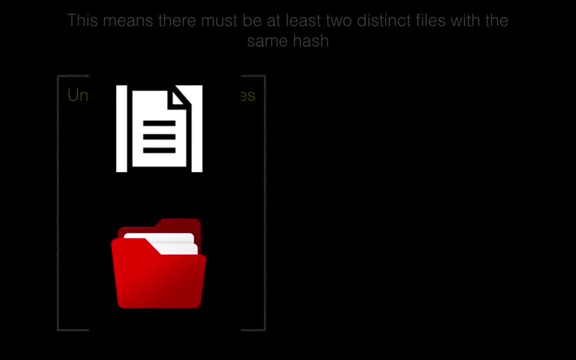 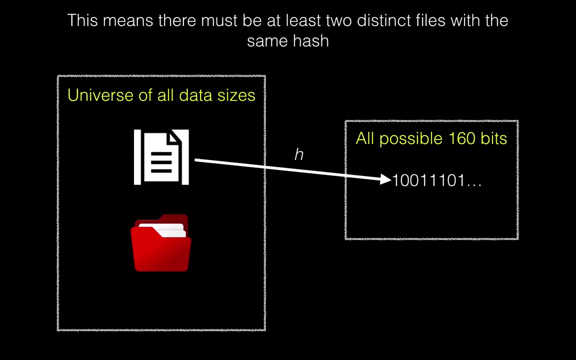 so, for example, i have these two files here, the white file and the red file, which could be a text file or a picture or whatever you want. so there must be two files that will have uh, if i apply h, whatever my uh function h- here the hash function gives me 160 bits, and this other file 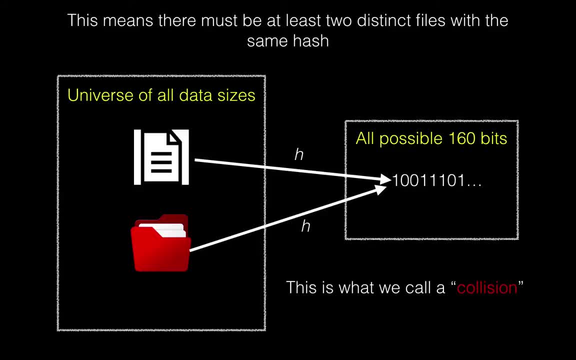 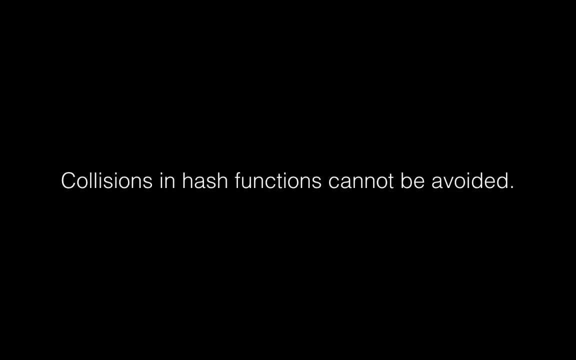 will have exactly the same output. so two inputs, two distinct inputs, will have exactly the same output, the same 160 bit output. that's what is called a collision, so a collision of a hash function. now the problem is, it doesn't matter how much you try, collisions and hash functions cannot be avoided, and the reason for that is: 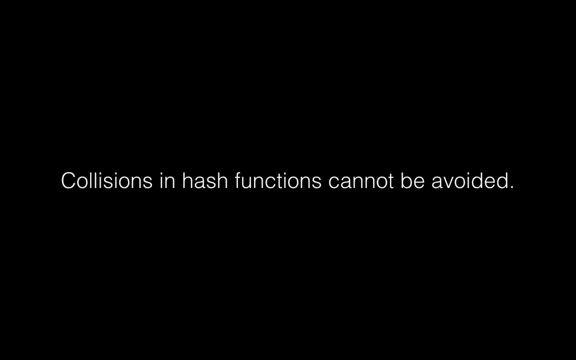 because the number of inputs is a lot larger than the number of output, because that's the design of the hash function. you want the output to be a fixed size, which is a smaller size. now you can think about collision in the following way: so let's think about it this way. so 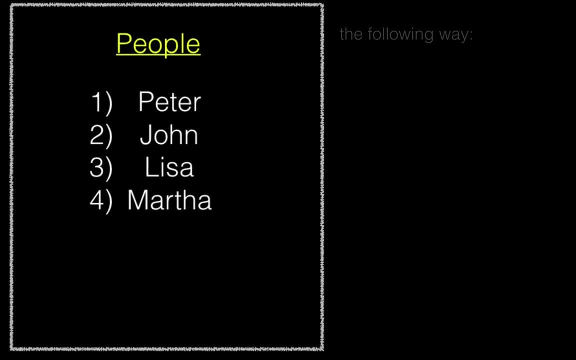 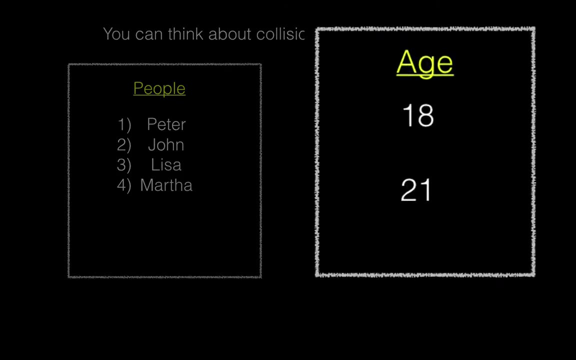 suppose you have the set of all people, whether they are, let's say, alive people in the world. so let's say we have example here: peter, john, lisa and martha, and that's going to be your inputs. now the output will be the age of people. of course there are more people than possible ages. 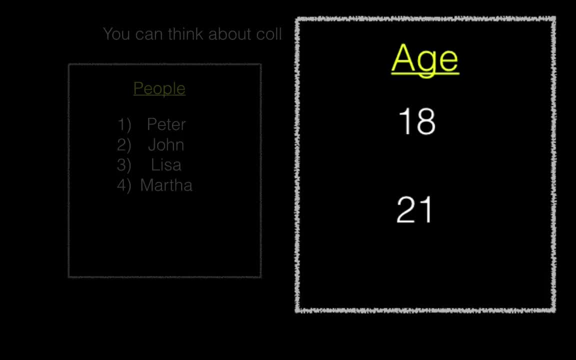 of course. so ages. if you think about of the standards, so you can have between zero and maybe between zero and 130 maximum. it would be very difficult to find someone who is as old as 130, but let's suppose it is like that. so the number of people 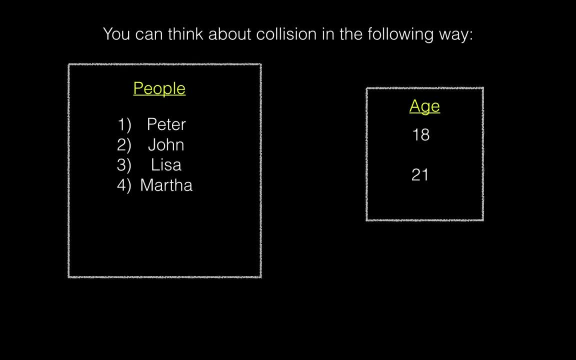 is, of course, a lot larger than the numbers between 0 and 130.. so there's bound to be collisions, if you think about it, of course, that always happens, so you always have people who have. for example, in this particular case, peter and lisa will have, for example, 21, are 21 years old and 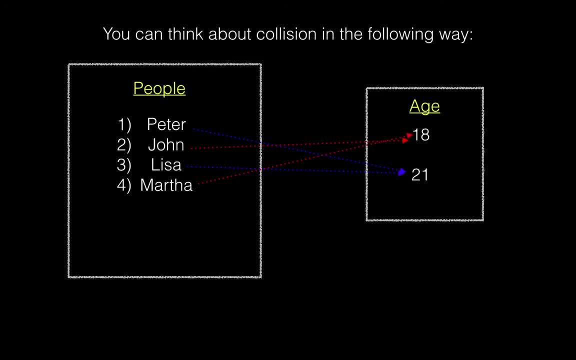 john and martha could have 18.. so that is a collision. and the reason you have a collision is because the number of people is a lot larger than the possible ages of people. so that's why the hash functions always will have a collision, no matter how you try to define it, as long as your 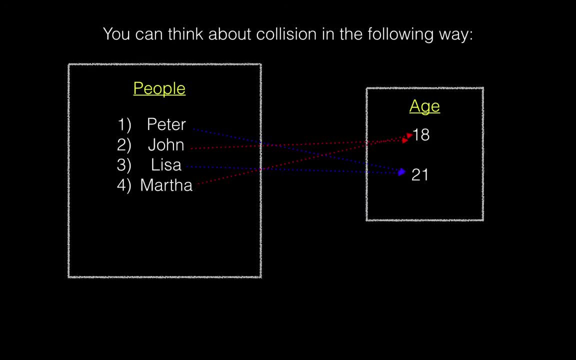 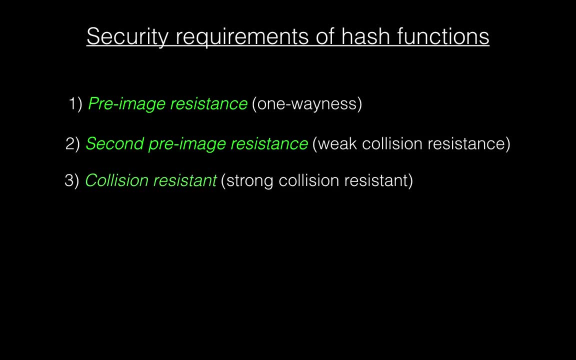 output size is smaller than the number of elements in your input set. so you always have collisions. so remember, these are the. so remember these are the security requirements. so we talked about number one, which is, uh, one wayness, and the two and three that have that word collision. so let's just go over two and three now. 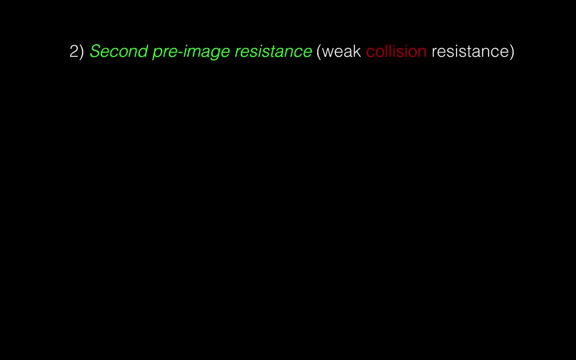 so two, which is the second pre-image resistance, but what we also call with collision resistance. so what is that? so suppose i suppose somebody gives, or an attacker has an input, given an input and an output, and of course the attacker also will have the information about what the hash function does. so the second pre-image resistance says that, because we already 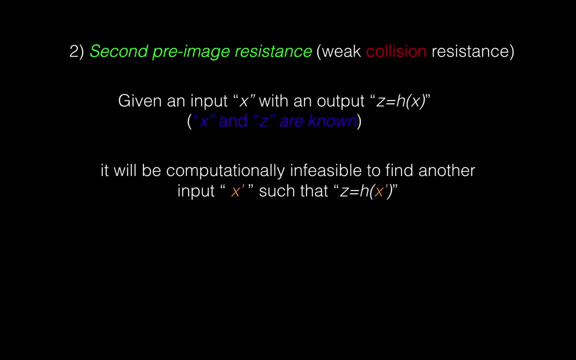 know that these things have collisions. then there must be another uh input. let's call it x prime. that will map to the output. now the second pre-image resistance says that finding that input is computationally infeasible. okay, let me explain that with a picture. so let's say you are. 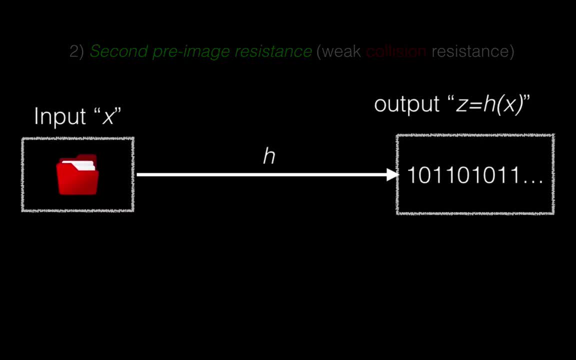 given this information here that i have uh here in the slide, so i have the output. so i know the output. i also know the hash function, or what the hash function does, and i also know the input. so i know the file in red goes to the output that you see there in binary now, because all hash 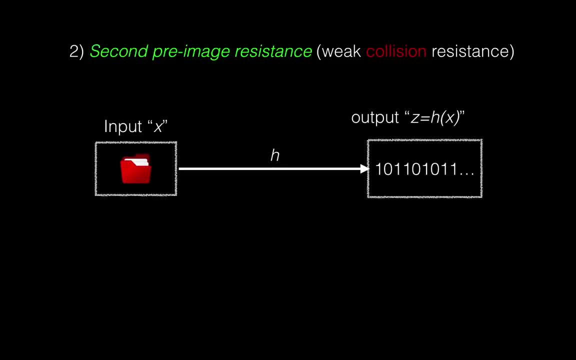 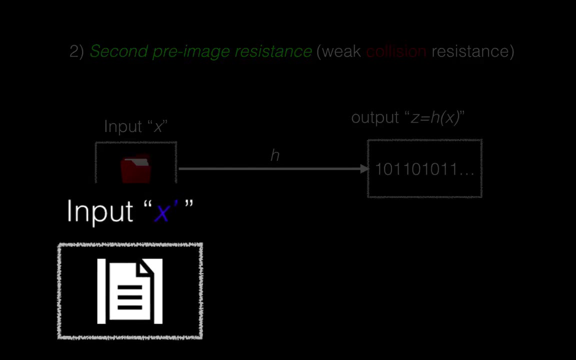 functions have collisions. i know there is another file that maps into that one, so and that's okay. the second pre-image resistance says that the design of the hash function, it should be such that if finding that other file, call it x prime, will be really difficult or will be computationally. 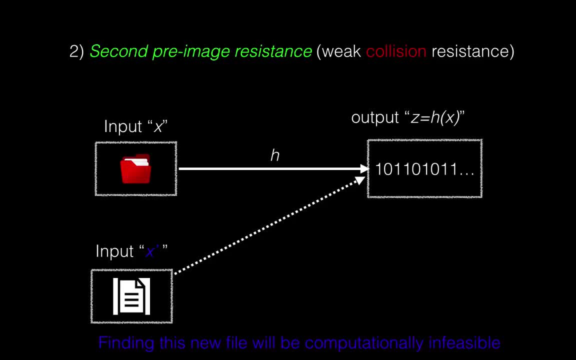 infeasible to find that other file. so that is the second pre-image resistance. now, all these security requirements i'm talking about, they have implications in on the way that the hash functions are used. so we talk about why hash functions have this kind of security requirements. later, 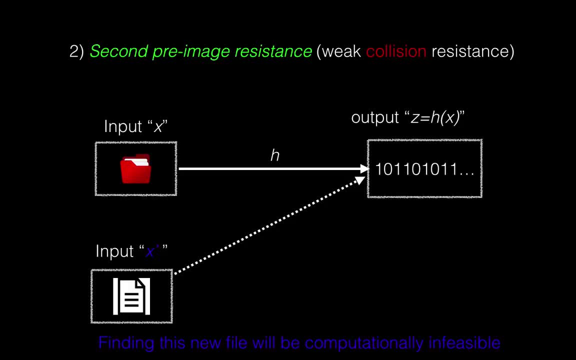 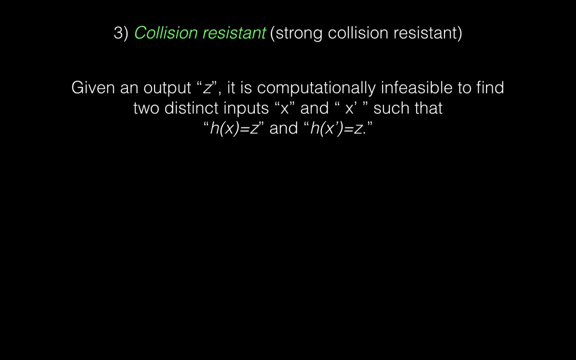 so not in this video. in another video i'll explain why this this is important to have. so that's the second pre-image resistance. now the third requirement, the third security requirement is collision resistant or a strong collision resistance. in this case, what you are given is the following thing: you have the output, and so it will be computationally infeasible to find. 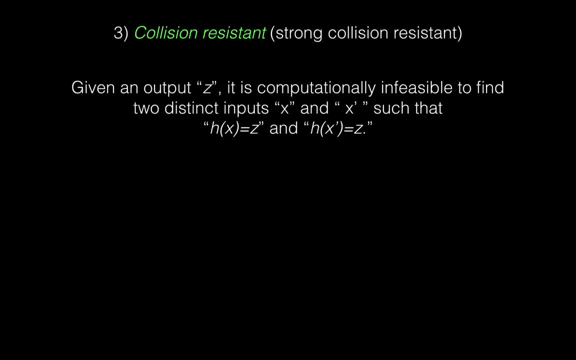 two hash functions that are in the hash function and the hash function that are in the hash function, distance inputs that go to the same output. remember this is talking about again collisions. in this case you are given less information that in number two. so in number two you have an input. 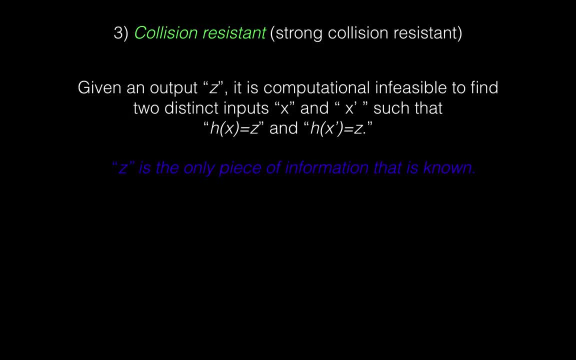 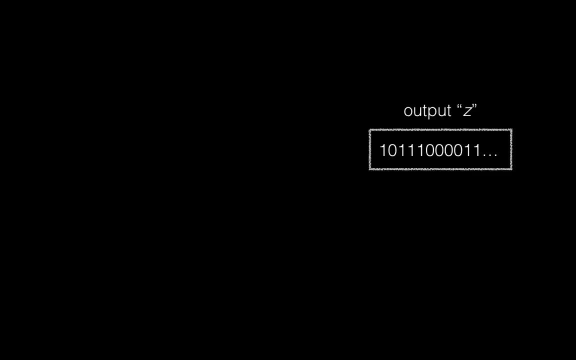 output and the hash function. in this case, you only have the piece of information. you have here is only the output and, of course, the hash function. so let's talk about that. so suppose somebody gives you an output, which is that binary number that you see there, uh, and you also have.